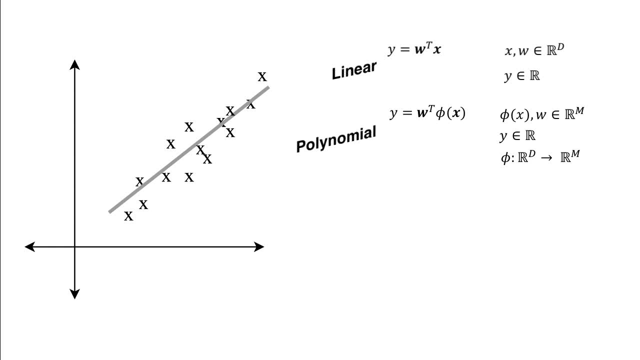 Note: polynomial regression isn't the same as non-linear regression. Phi of x is just square terms, cube terms and polynomial terms in general. With this we can create complex models. But how do we find phi of x Simple? Normally without the basis function and just considering the base features. 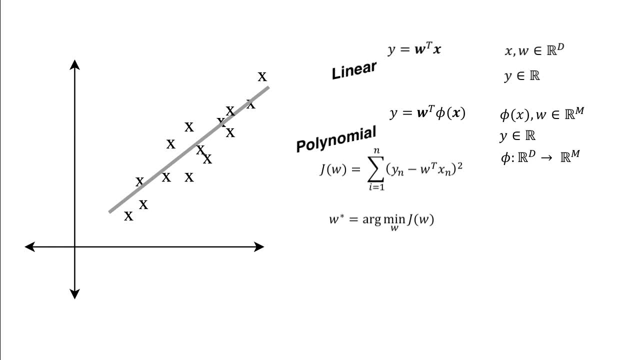 we minimize the least-squarest cost function with respect to the weights. After vectorizing and simplifying you get optimal values as x transpose x, the whole inverse times x transpose y. I made a detailed simplification of this in my linear regression video. 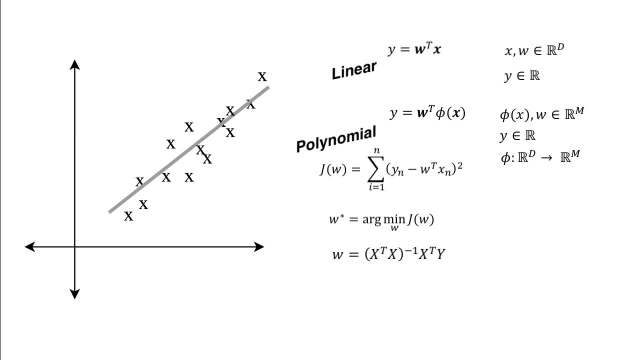 so check that out after this one. Now what we want is the weights for the non-linear basis function. So replace x with phi. Want to include regularization, Just include lambda. i- Lambda is the regularization parameter and i is the identity matrix- With else regularization. this is now ridge regression. 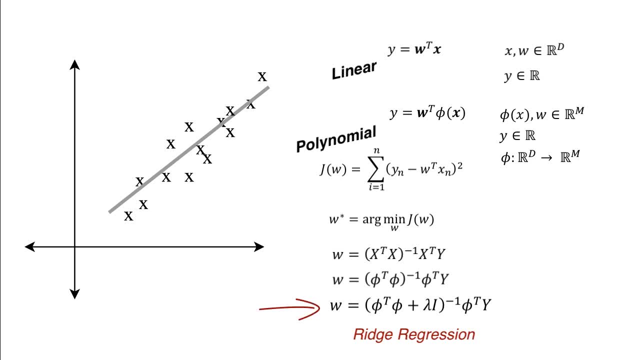 The point of a parametric model is to estimate the value of parameters, which we can do only if we know phi, Or at least the covariance matrix. phi transpose phi. But that's pretty hard to compute. so you can clearly see the problem here. 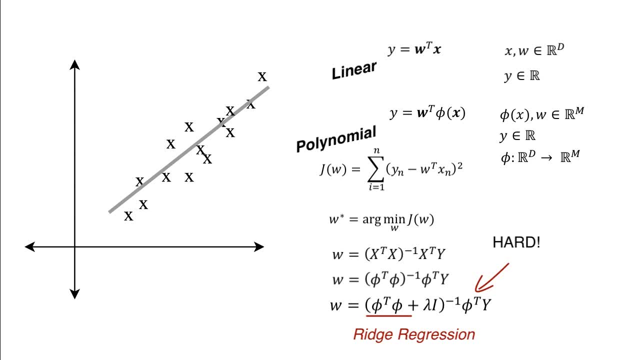 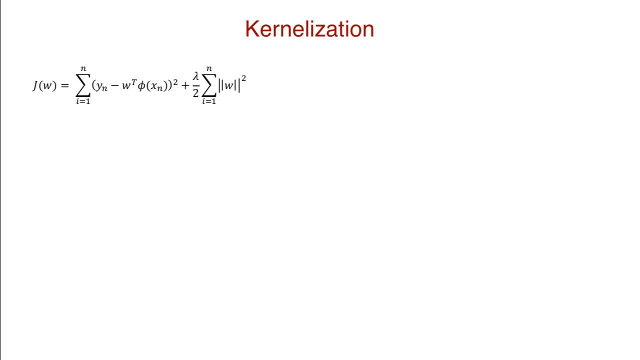 We're going to do this entire thing again, but this time with kernelization. So consider our ridge regression cost function j, Taking the derivative with respect to the weight vector and equating it to zero, we solve for w. To make things easier to look at, we'll call the first part alpha. 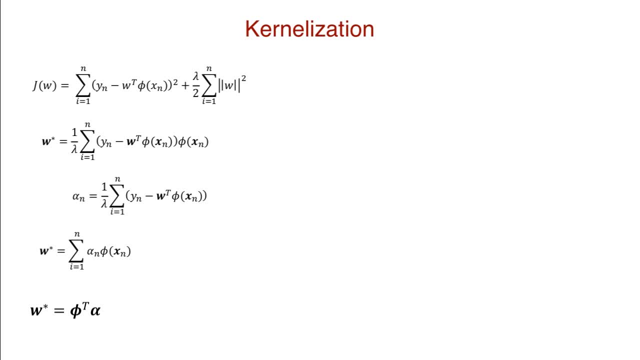 So the weights become the dot product of the basis function and alpha. Once again consider the original cost function and vectorize and substitute our weight w. Then we just keep simplifying. The repeated term is phi, phi transpose, which is a square matrix called the gram matrix or kernel. 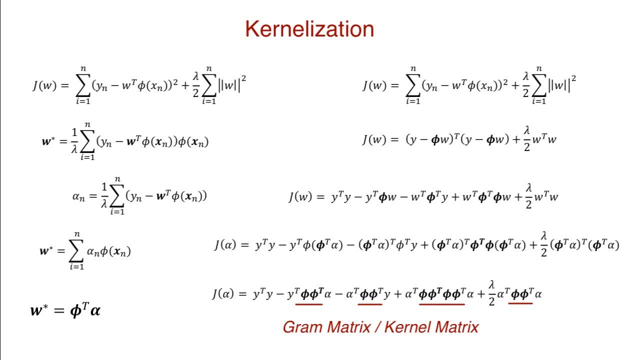 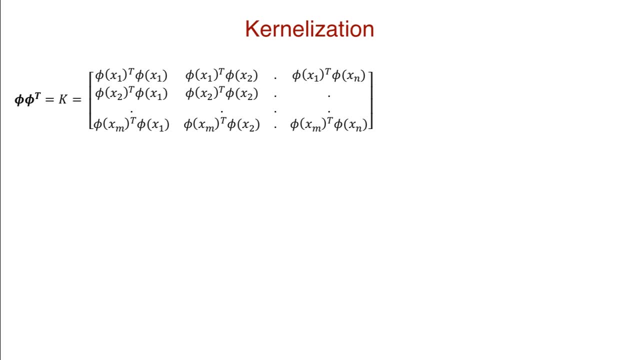 matrix denoted by k. So the term is phi phi transpose, which is the square matrix called the gram matrix or kernel matrix denoted by k. Now we're getting to the juicy stuff. The kernel matrix, phi phi transpose, has elements that are the dot products for every pair of feature vectors. 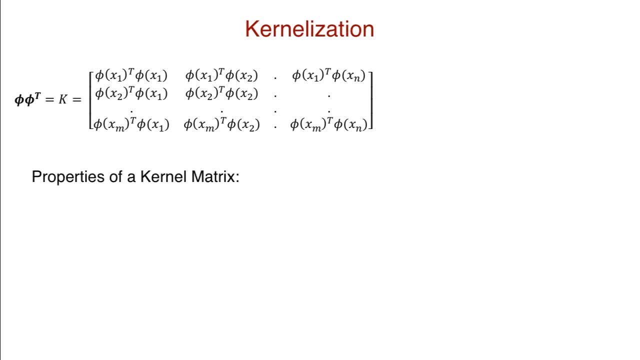 This kernel matrix is of significance because of two properties: It's symmetric, so the matrix equals its transpose, And two, the kernel matrix is positive, semi-definite, so the product with any other vector and its transpose leads to interval, a non-negative solution. 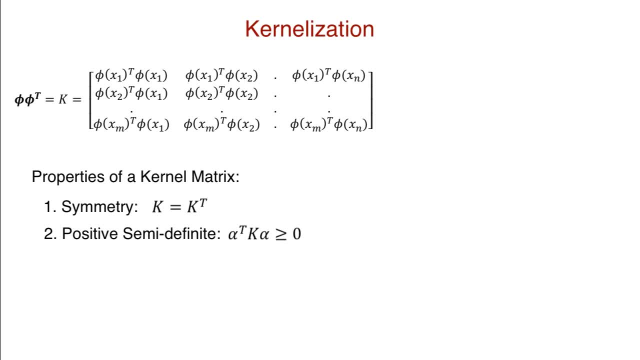 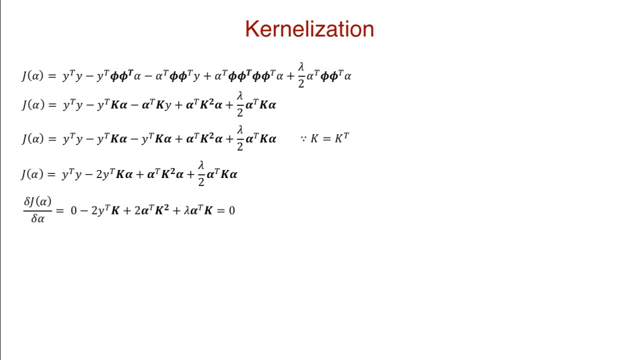 I'll come back to why these properties are important in a bit, but for now let's use these properties in our simplification of the cost function. First off, transpose the scalar term. We can do this because scalars are symmetric. We minimize this cost function to get the optimal value of alpha. 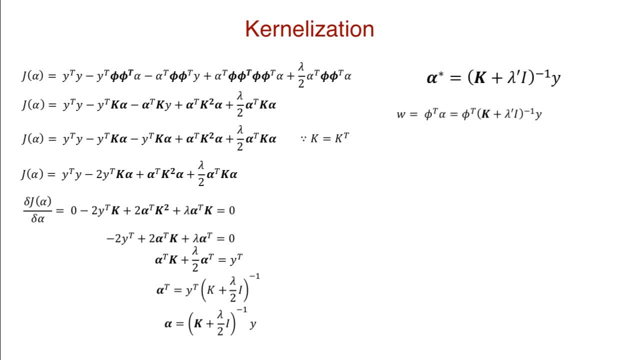 Once we have the optimal alpha, we can express the weights in terms of this kernel matrix. So what's the difference between this set of weights and the one that we computed before, without kernels? Before we had to compute phi, transpose phi, which is the covariance matrix, but now we 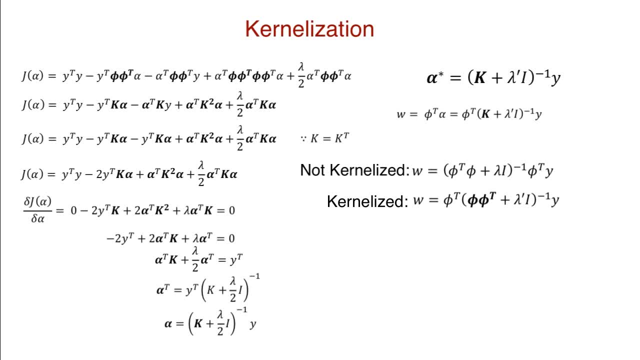 need phi. phi transpose the kernel matrix, But wait, it looks like to compute this inner product as well. we still need phi. However, that's actually not the case. I said before, this kernel matrix has two properties. One is that it's symmetric and two is that it's positive, semi-definite. 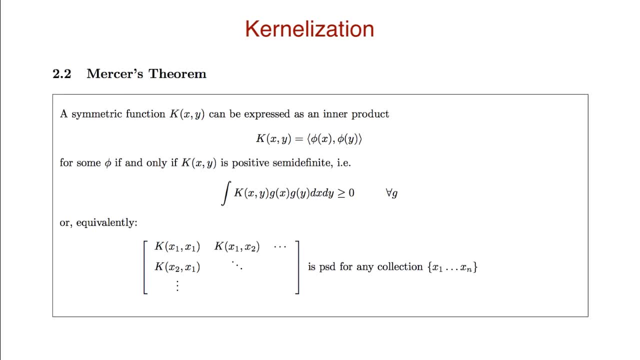 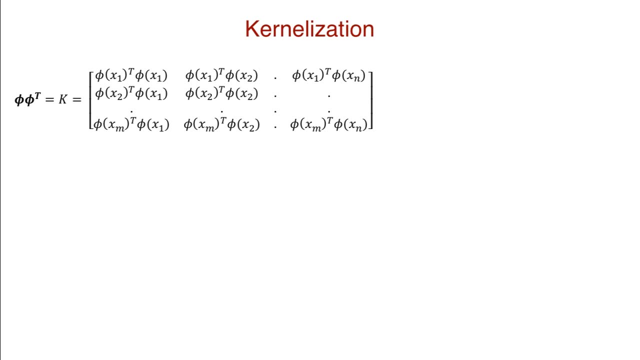 According to Mercer's theorem, a symmetric, positive, semi-definite function can be expressed as the inner product of some phi. In other words, we can rewrite every term in the Gram matrix such that it is a function of only the base features. This is the kernel trick and the fundamental reason why kernels are so powerful. 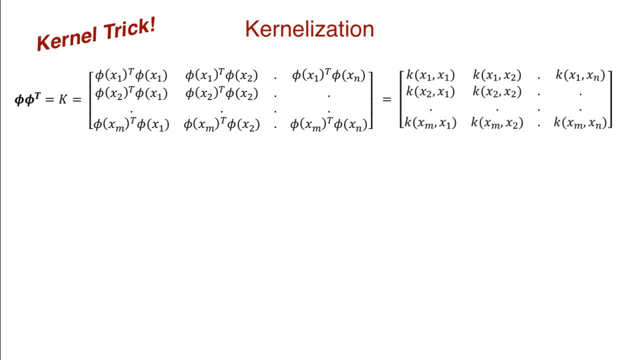 I'll show you with an example of how this kernel trick works. Consider this polynomial non-linear basis function. We have the kernel matrix where every term is an inner product of two samples. Expanding these terms, we can see that this inner product of non-linear basis functions. 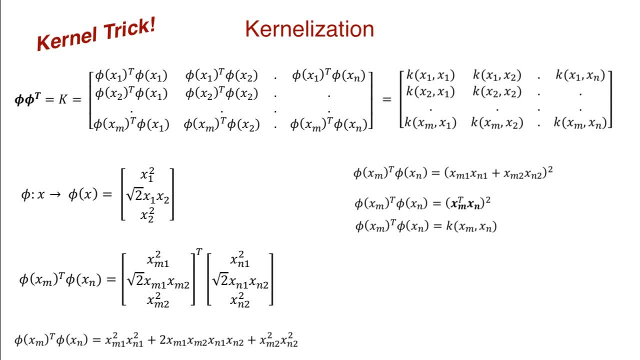 can be represented as a function of the basis vector inputs xm and xs. This is the kernel trick and the fundamental reason why kernels are so powerful. I'll show you with an example of how this kernel trick works. Expanding these terms, we can see that this kernel trick works.